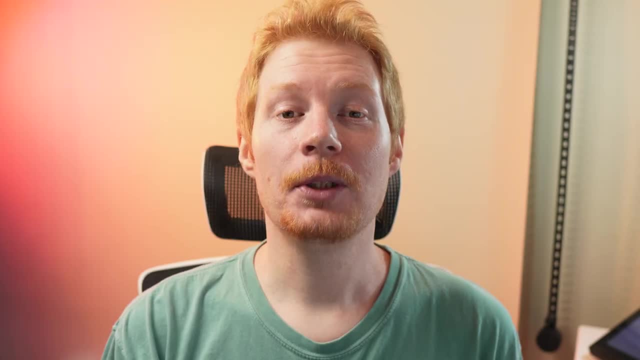 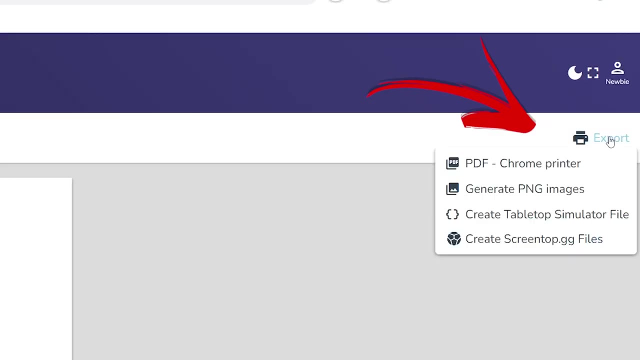 Let me introduce you to level four. Dexterous is a website that you can use to manage your game project. It allows you to set up card layouts, so you don't need to design and make changes to each individual file. One feature that makes this so special is the ability to 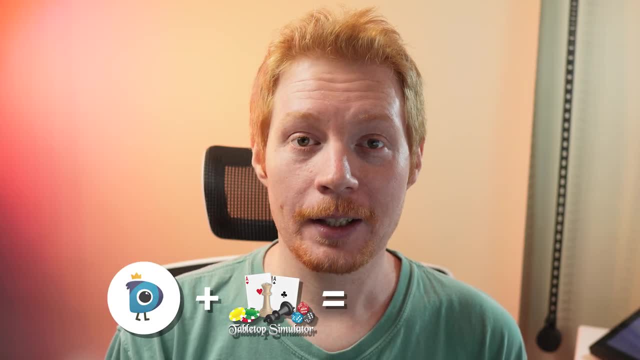 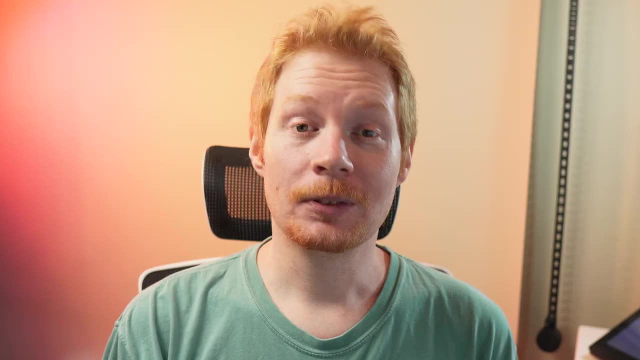 export that project Dexterous, paired with something like Tabletop Simulator, allows you to make changes and play your game incredibly quickly. But we're not stopping there. In this video, I'll walk you through what you need to reach level five. 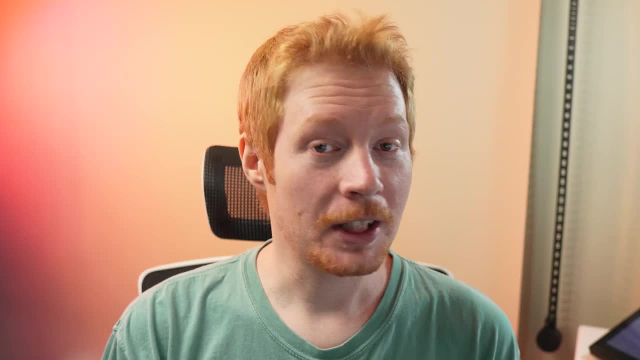 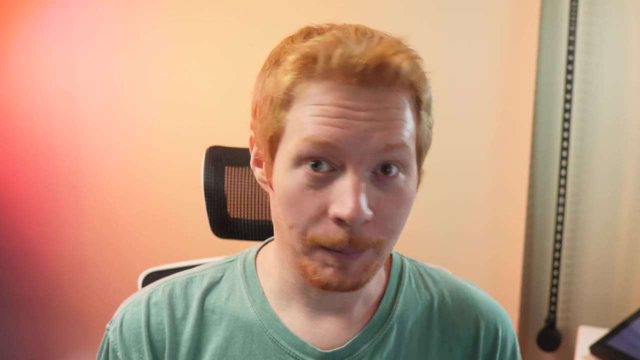 where you and as many others as you'd like can make as many sweeping changes as quickly as you'd like. that will update every single card and token in your game near instantly. I want to show you what this looks like immediately, so check this out. So, as you can see here, this is one of the 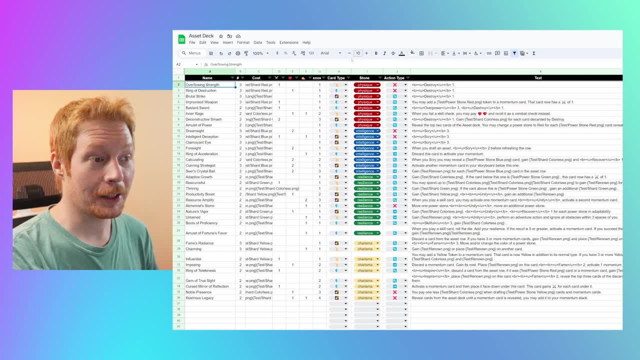 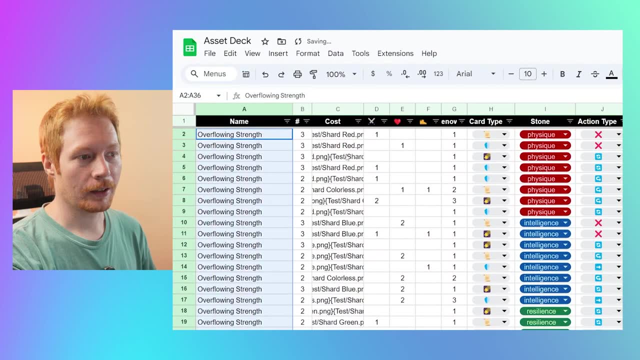 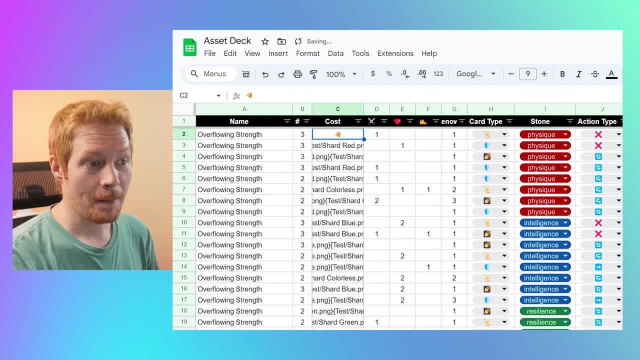 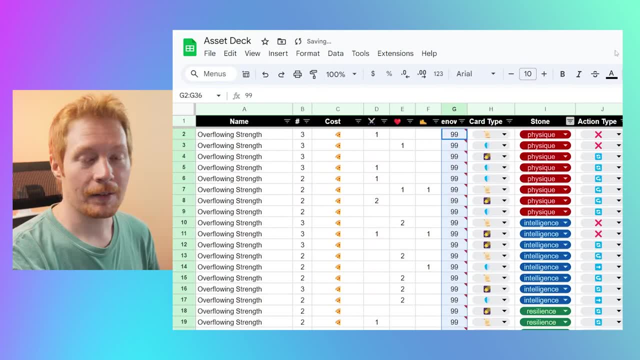 And we like the idea of everything costing a single slice of pizza. And then, lastly, the point values were pretty low and we really think that the best way to move forward is to make everything worth 99 points, And as quickly as that, we are able to go play test all of these. 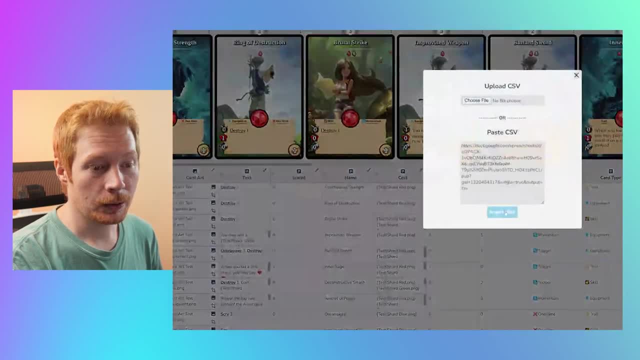 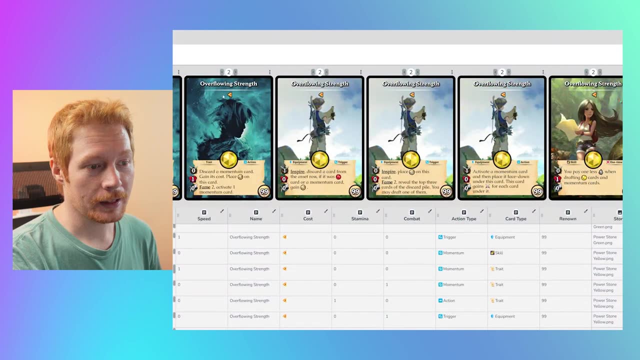 changes Come over into Dexterous and we tell it to refresh the data and update to all the changes that we just made. You can see that everything is now called overflowing. strength costs one slice of pizza and is worth 99 points. 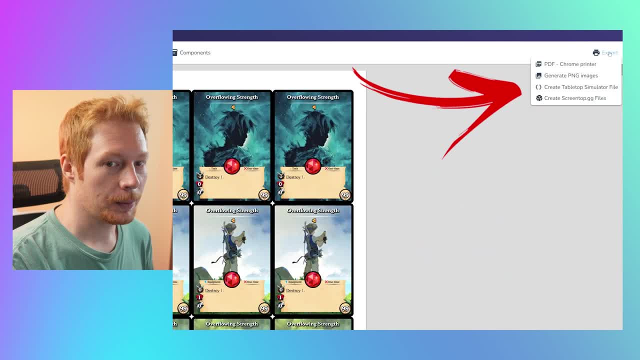 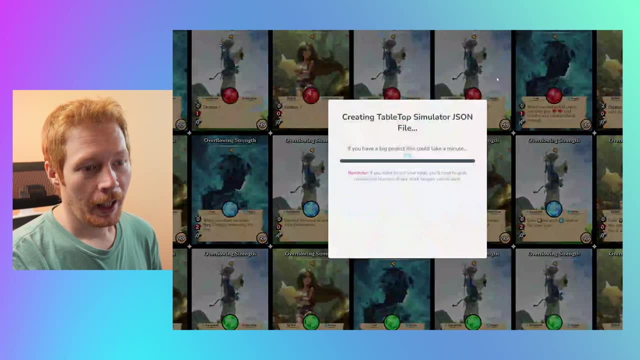 Next thing we need to do is export this and tell Tabletop Simulator to update its information to the new changes. You give it just a couple of moments. it runs through a loading bar and as quickly as that we are able to jump into Tabletop Simulator. 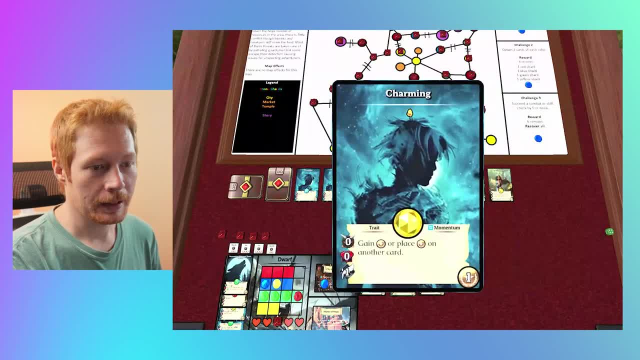 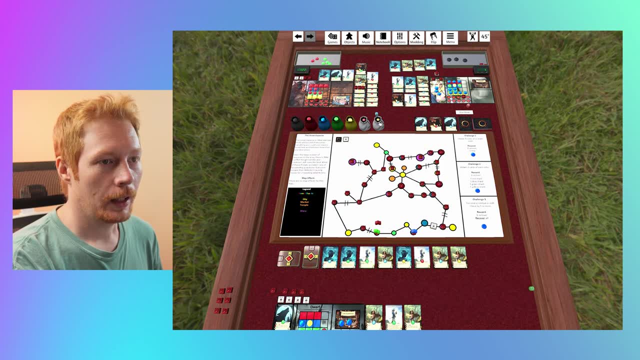 So this is a snapshot of one of our games recently played and you can see that all the cards are still individually named, have different costs and are worth one to four points. Now we want to play test our changes, So we go back to the main menu and that part's actually. 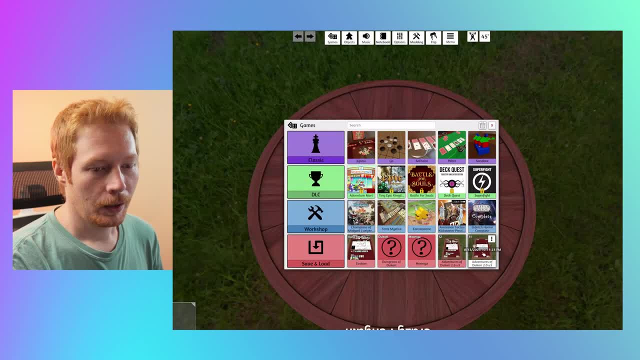 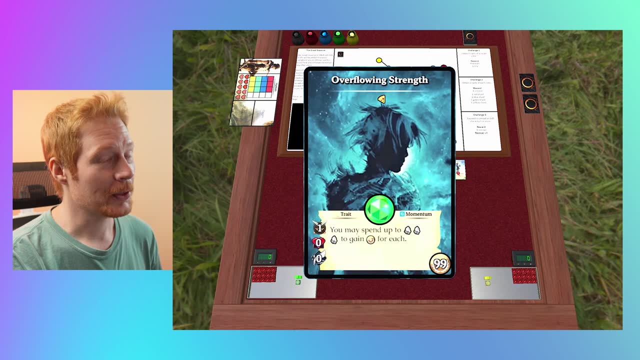 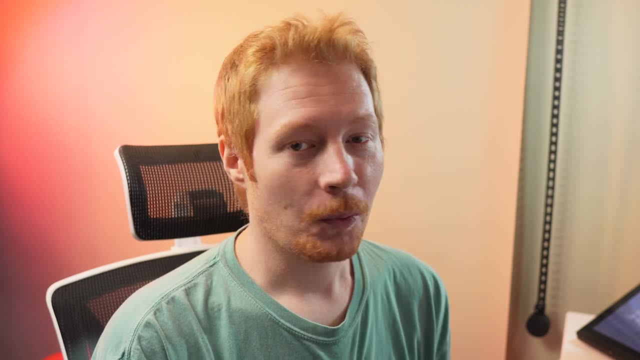 called Overflowing Strength, and I'll explain that later. Let's create ourselves a new game, and as quickly as this, we can now see that everything is called Overflowing Strength, costs one slice of pizza and is worth 99 points. There was a time when I would make all of those. 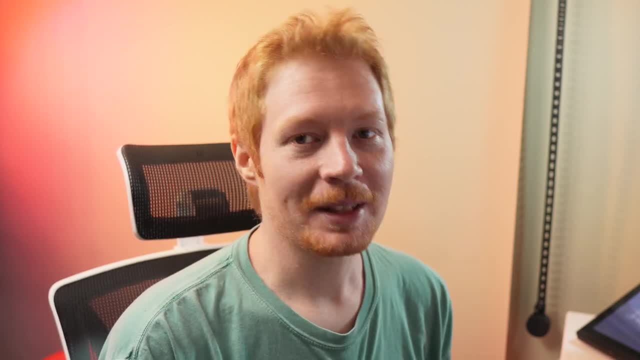 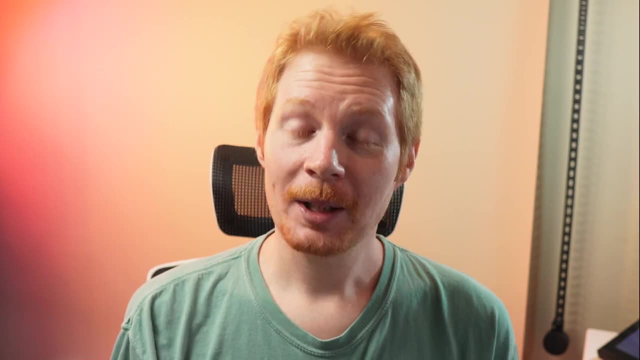 changes one page, each card at a time, one image, one text field. This is the difference between level three and level five. Hi, my name is Dave Geltema. Welcome to Tabletop Craft, where I help newbie game designers learn their craft. In this video, I will walk you through. 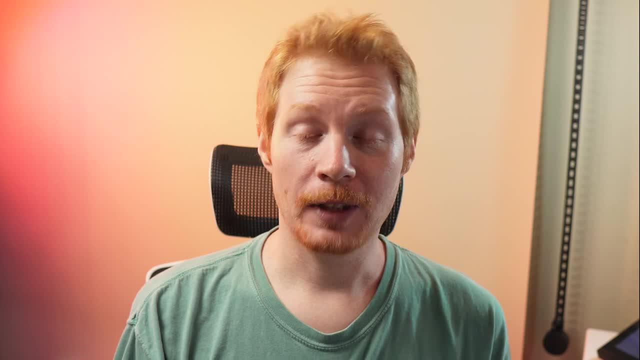 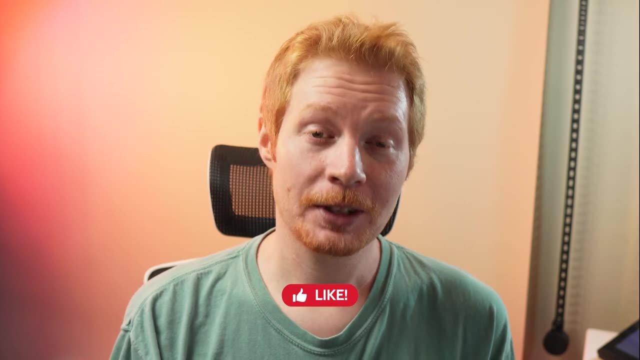 step-by-step on how to use dexterous and why it's a game changer for rapidly prototyping. If, at any point, you find any of this information helpful, I'd appreciate it if you hit the like button or if you just feel like helping me out so this video has a better chance to reach other. 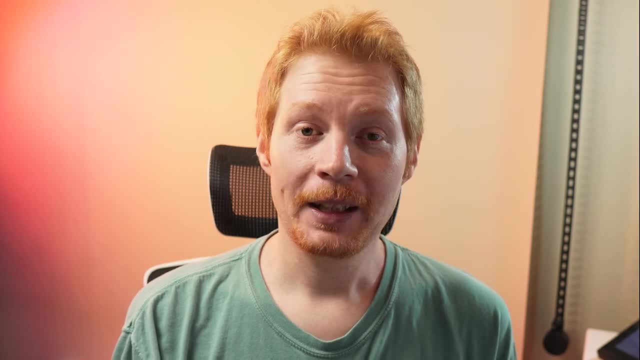 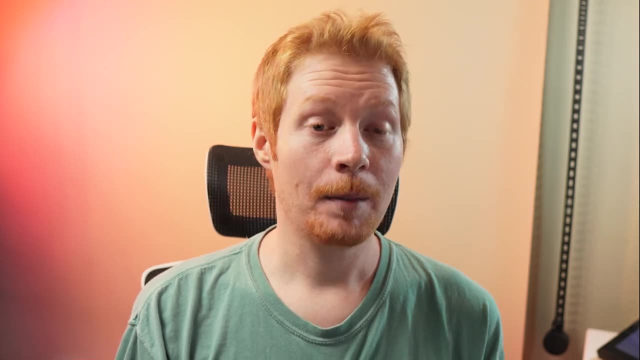 people. that like button really does wonders. Recently, my buddy and I went back to the drawing board for our game, but by using the tools and method in this video, we were able to rapidly prototype and play test our game into a very good spot in just about a month and a half. 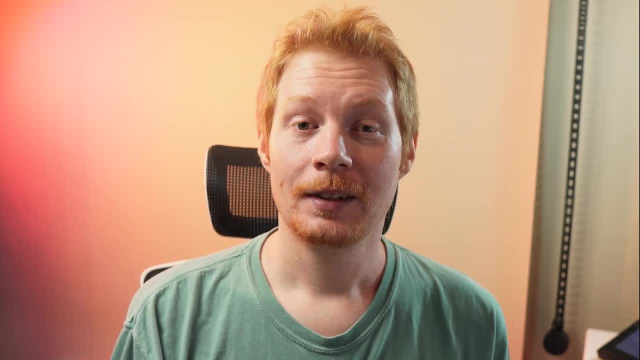 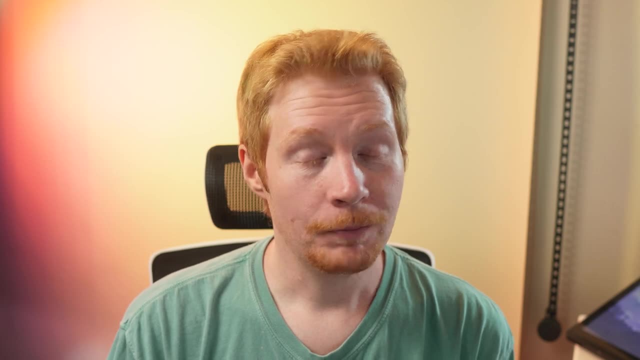 All right. so what do you need to do this? Let's walk you through the steps. Step one: create a dexterous account. You want to make a game, something you can rapidly prototype and play? test at lightning speed. Use dexterous. Simply go to their site and create an account. The free tier is more than enough to do everything you'll need. Once you've created your account, you need to make a new project, So go to the project page and hit the plus sign to create a new one. In the top left you can give it a name. 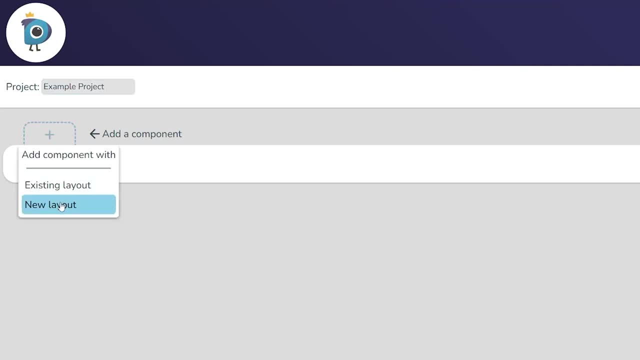 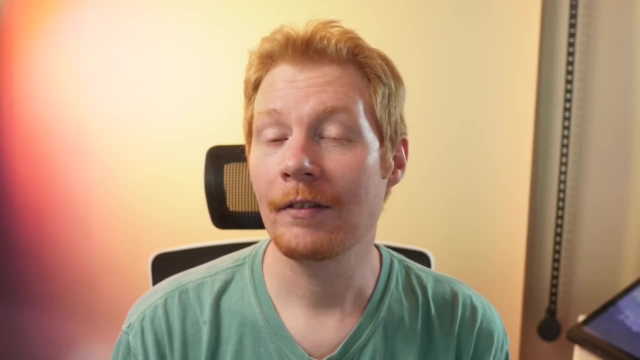 Start by adding a component, but each component needs a layout, so select the new layout option. A layout is a template for a component. Imagine a set of cards or tokens in your game that all have the same format. You can make more. The interface is fairly self-explanatory On the left side of 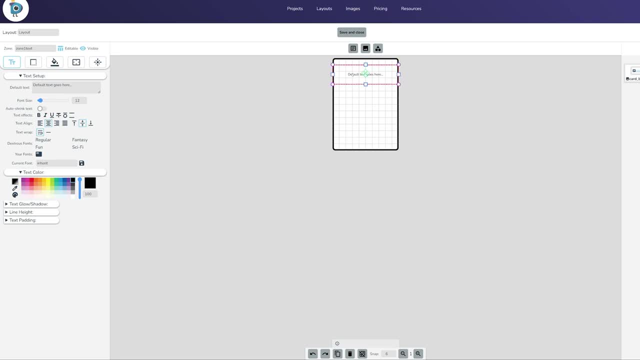 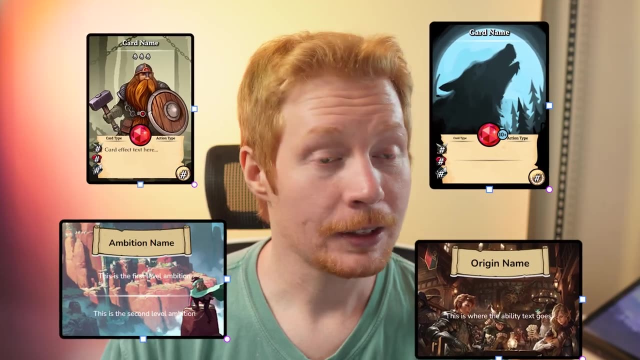 the screen. you can import images and control the size of text Across the top. you can create layers and you see them in the list on the right. Here's a few examples from our game. You can play around in here as long as you'd like, or you can make a simple card and come. 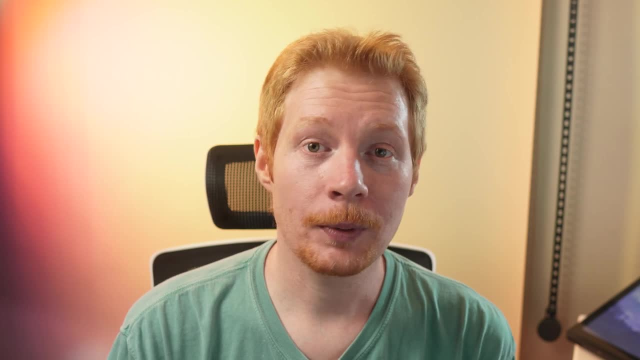 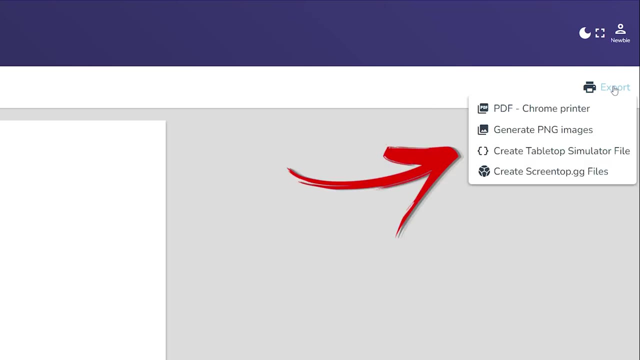 back to make it look pretty later. At any time, you can export your cards to be printed or, better and more importantly, you can export as a tabletop simulator file. This allows you to load all of your components at once into TTS so you can play virtually with your friends on Steam. 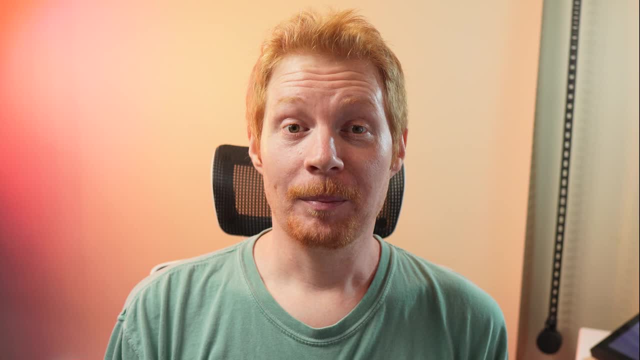 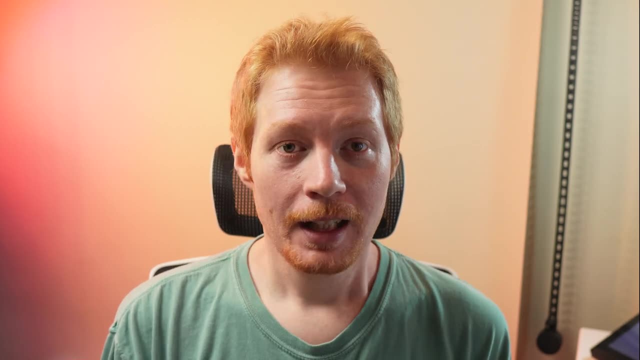 Step 2. Tabletop Simulator. So you're making a game, but you need to playtest it. I think that playtesting your game digitally is the way to go When it comes to rapid prototyping and playtesting. it is infinitely easier to get your friends together to play your game online. 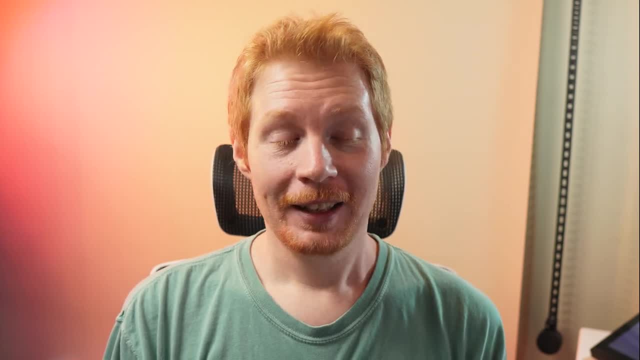 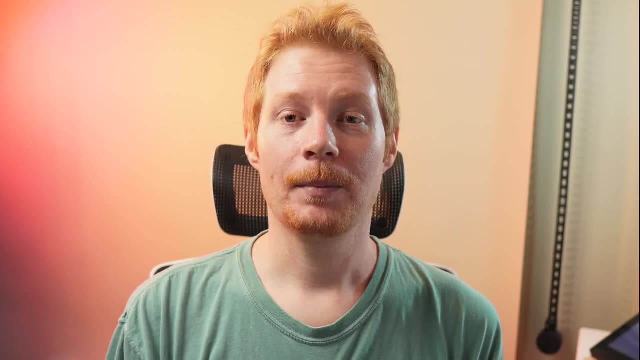 than it is in person. I should know I've run D&D 5e. It's also infinitely easier for strangers to try it out digitally as well. Tabletop Simulator is my platform of choice to playtest my games. It is a virtual tabletop where you can play and do pretty much anything you can think of. 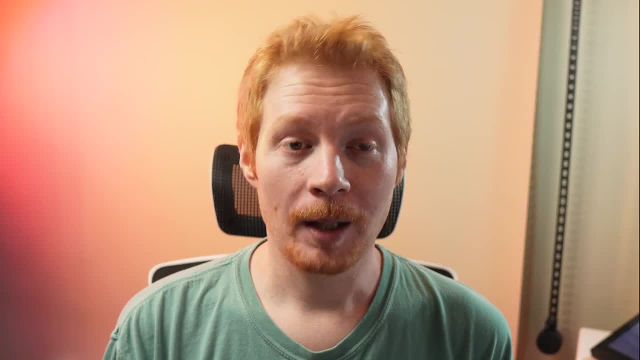 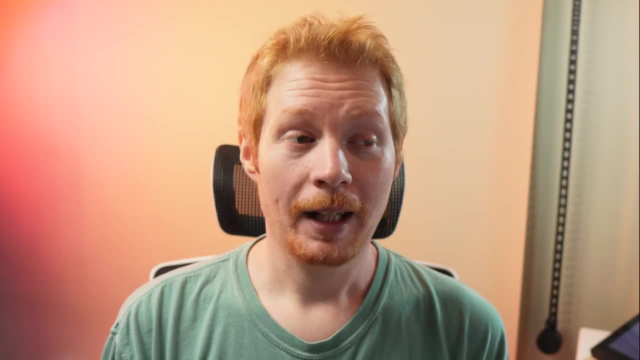 It's a community-driven game that costs $20 on Steam, where people have uploaded every board game I've ever thought to look up. It's a great platform to play games, which makes it a great platform to playtest games. Depending on how involved you wish to get, you can program just. 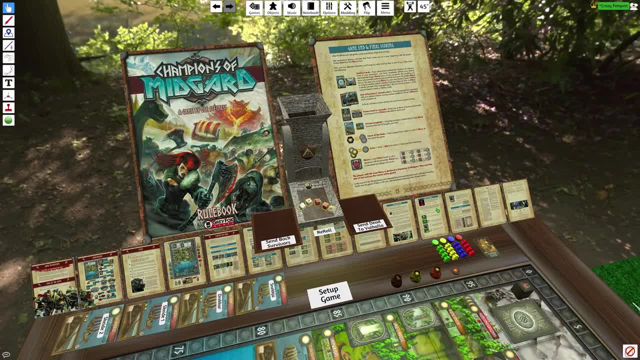 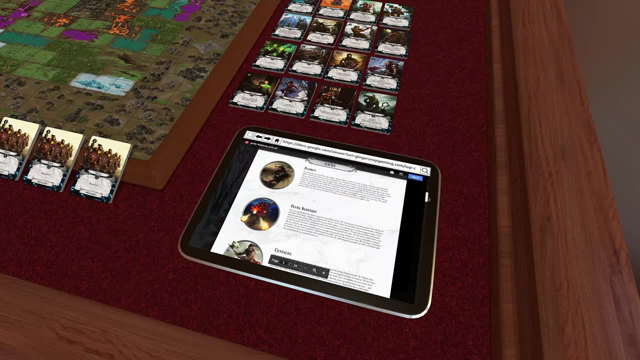 about anything you think of. You can import custom assets, automate games with scripting, automatically count resources. You can even place a virtual tabletop simulator on your tabletop simulator, a virtual tablet on the table that you can browse the web or open PDFs with. The sky's the limit. 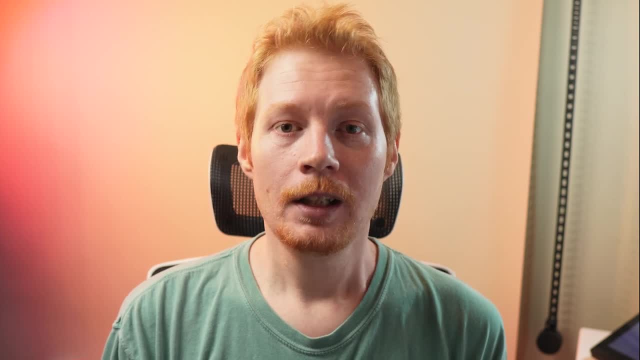 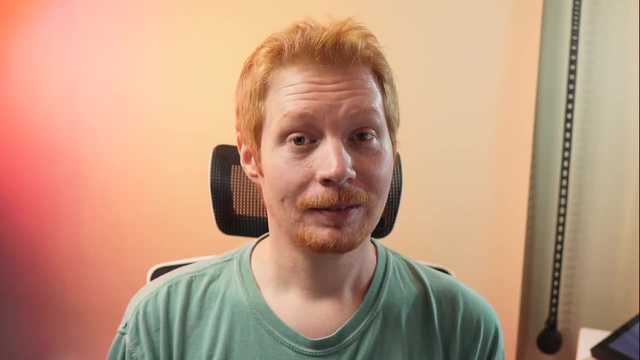 And, most importantly, when importing a dexterous project file, you have every component you've ever designed, instantly ready to be shuffled and used at a moment's notice. But we can take it even a step further. Step three: Google Sheets. When making a game, the best way to make sweeping 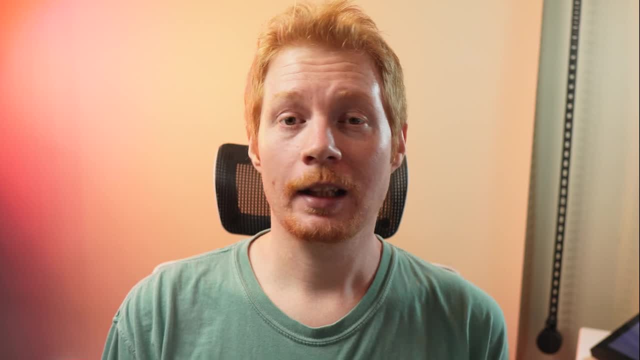 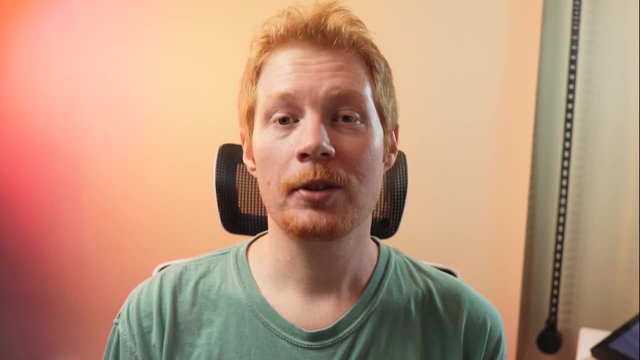 changes is through the use of spreadsheets. You can see everything at a glance because every value is right there, listed next to the others. You can compare the wording of effects side by side. change the VP values of every card all at once. make sure every card's name follows the same theme. 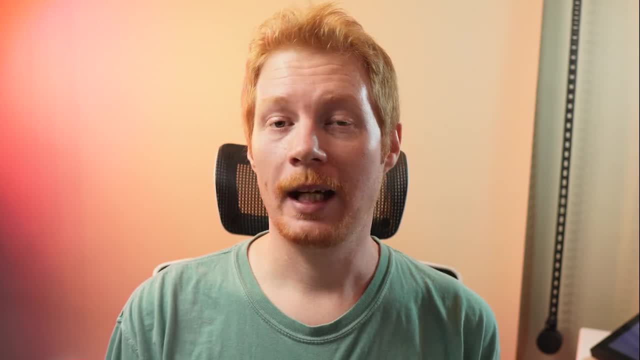 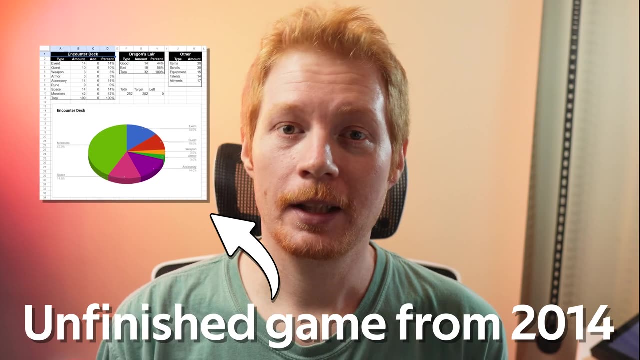 change how many of each card are in your game and sort by every variable you have. Spreadsheets allow you to take it a step further. You can set up reference pages for shorthand or you can make pie charts showing the percentage of card types and categories in your game. But I think the biggest 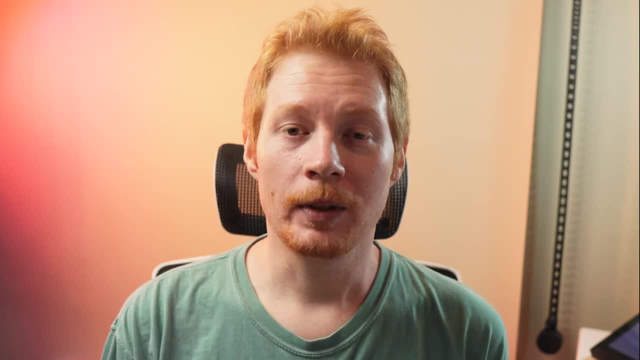 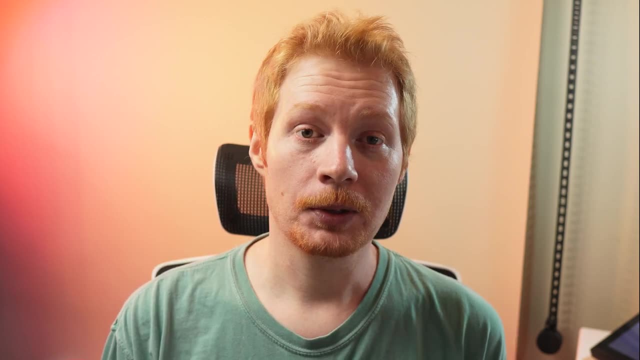 benefit of working on your game in Google Sheets is that you can edit with as many others at the same time as you'd like Most other platforms or methods. you're stuck working on each file individually. You can edit with as many others at the same time as you'd like Most other platforms or methods. you're stuck working on each file individually. 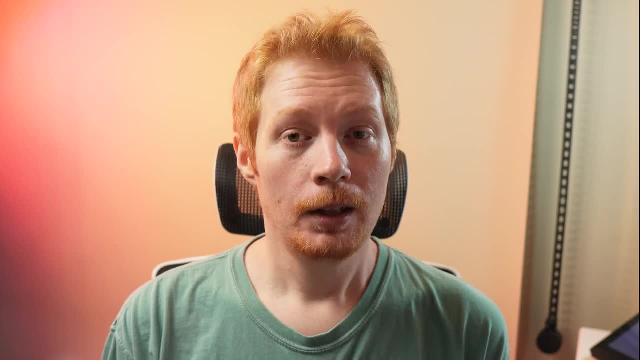 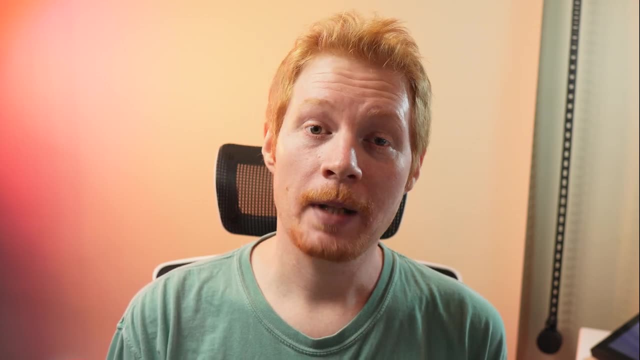 And if anyone else is helping you, you tend to overwrite each other's work. You can spend as much time as you want customizing your spreadsheet By publishing this to the web as a CSV. Dexterous can make all the changes you make here to all of your cards with a click of. 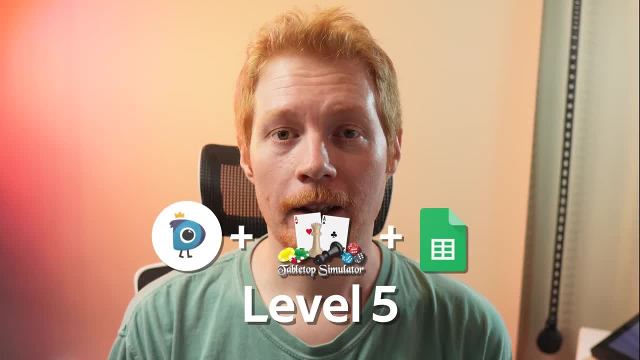 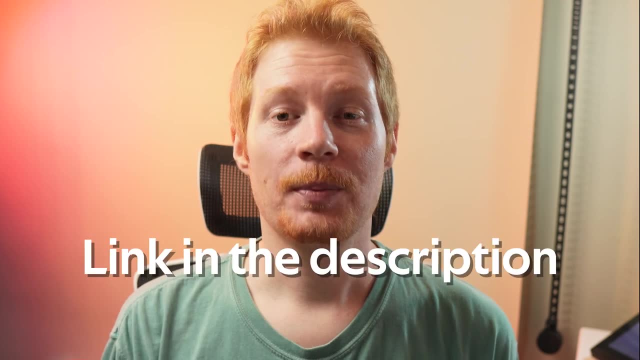 a button. When you have all three things- Dexterous Tabletop Simulator and Google Sheets- working together, it's like assembling each piece of Exodia. You win the game. If you want to try it out, there is a link in the description where I have provided everything. 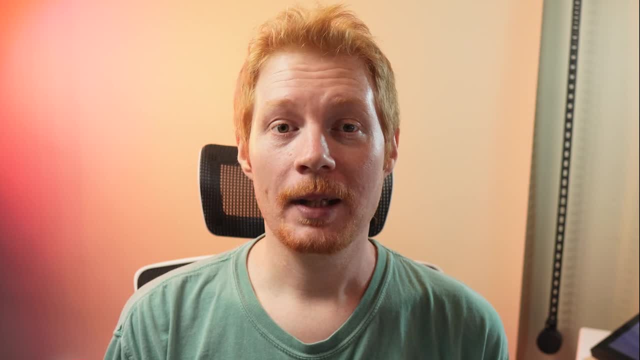 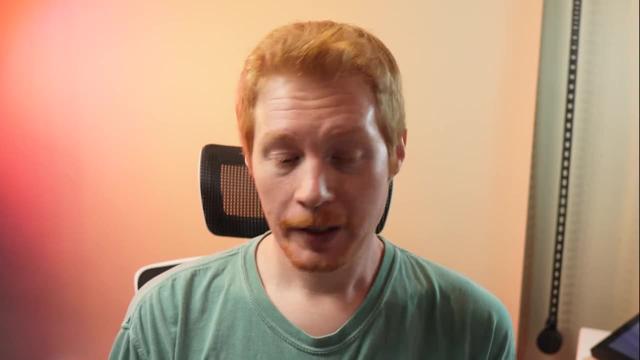 you need to do this yourself. It's a starter kit. It'll walk you through step by step to download a template Dexterous project with a link to a Google spreadsheet that you can copy for yourself that is linked to that Dexterous project. This way you can hit the ground running with most. 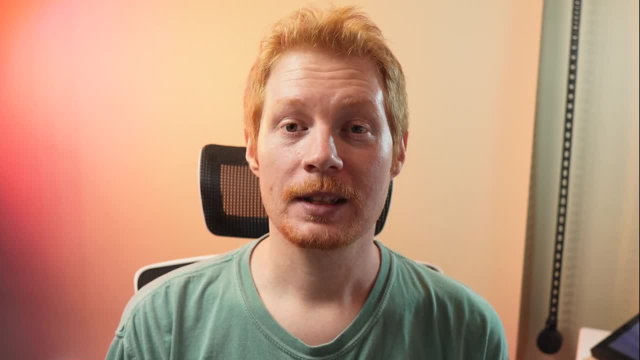 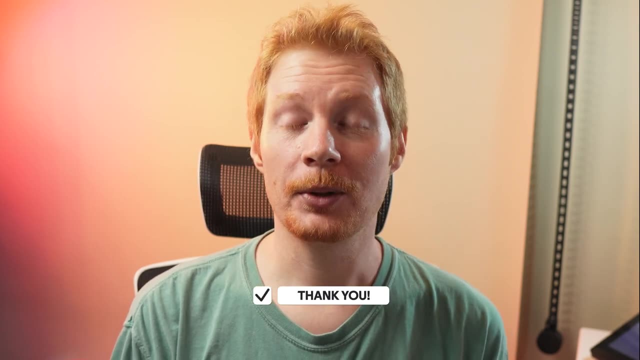 of the work already done for you. Feel free to reverse engineer it for your own purposes. If you are interested in more helpful tips for game design, be sure to hit that subscribe button so you don't miss when the next Tabletop Crack video is released. And there is one final step. 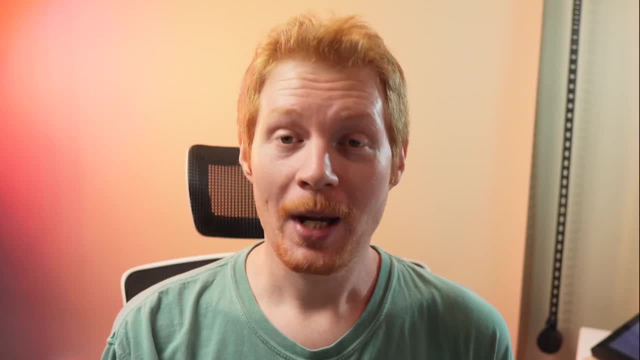 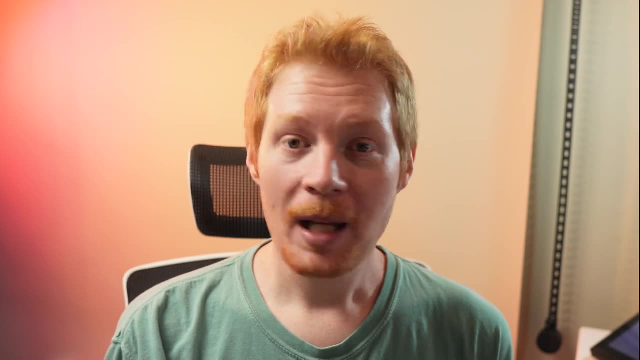 to follow. Step four: playtest. So you have your game in mind and a good idea on how to rapidly prototype it. Now you need to playtest. Go get some friends together and try it out. But maybe you could use some new friends or a fresh set of eyeballs to take. 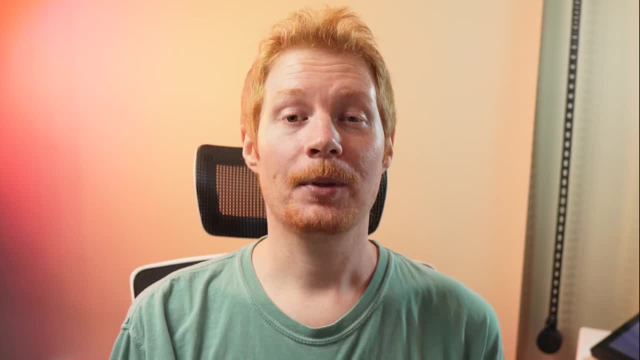 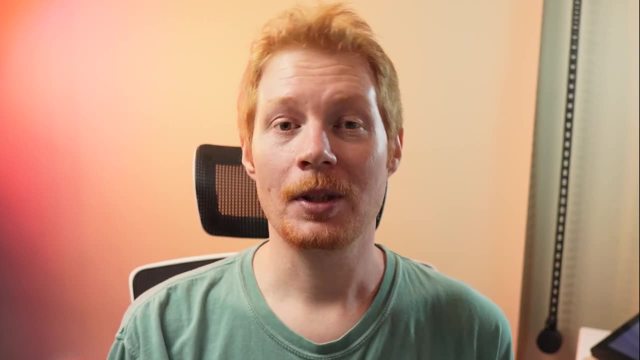 a look at your game. If that's the case, then you can come join me in the Tabletop Craft Discord. I'm starting a new community on Discord for beginner game designers and playtesters and I'm filling it out with all of the best resources I can find. All the lesser known tips. 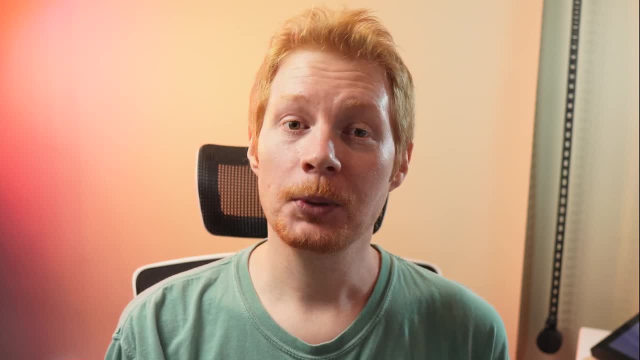 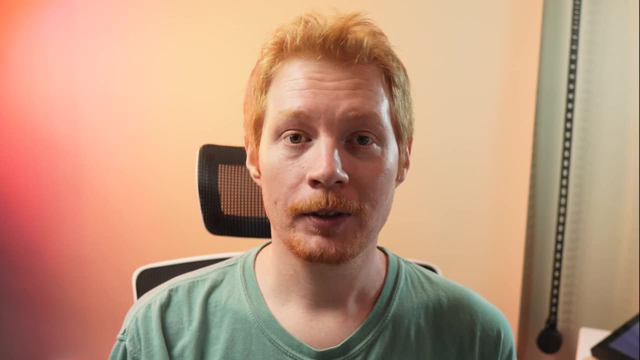 and tricks and best practices, like the method in this video. If that sounds cool, you can find a link to it in the description of this video. I think that this could be a cool place to gather like-minded people who you can bounce ideas off of and ask their opinion on specific questions. 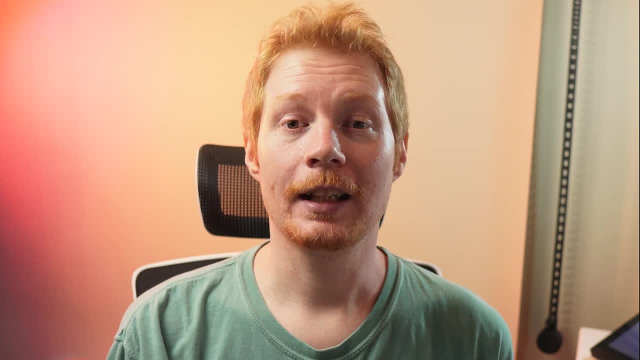 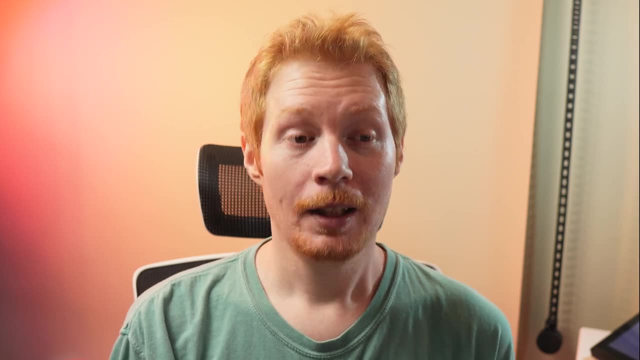 Help me build this community of game designers and playtesters by clicking the link in the description. Come say hi Once again. there is also a link in the description that you can follow to get a head start on how to do this for your game. Just know that I'm not your guy when it. 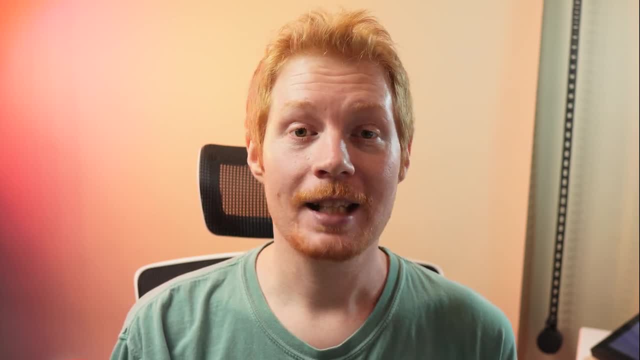 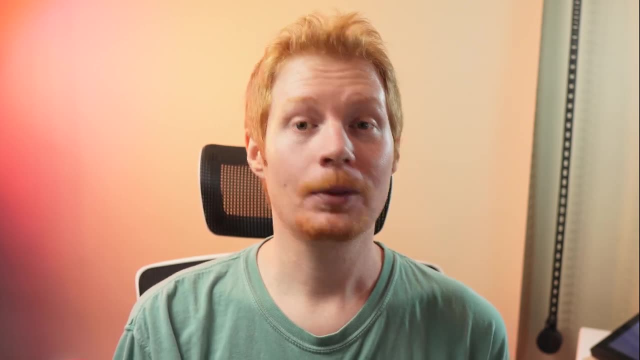 comes to specific technical questions, The Dexterous website has in-depth step-by-step video walkthroughs for you. if you learn best that way And if you have specific technical questions, the Dexterous Discord is the perfect place to ask them. Talk to the guys who made it. They're. 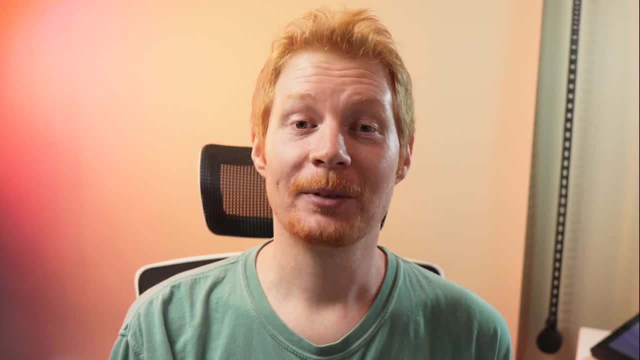 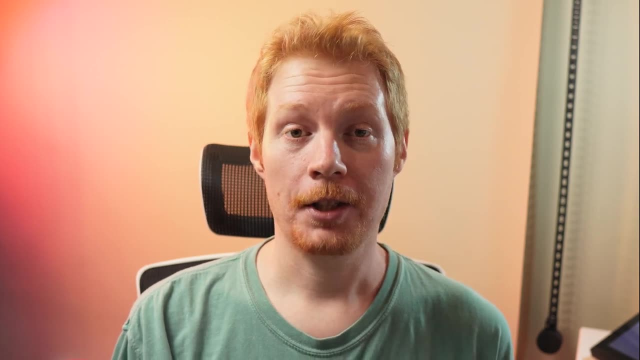 great at responding to questions, I hardly know enough to make this work in the first place, so go talk to them about how and why it works. A quick tip and a lesson learned: I would suggest turning off the mod caching option in Tabletop Simulator. This will save you a step each time you go to play. 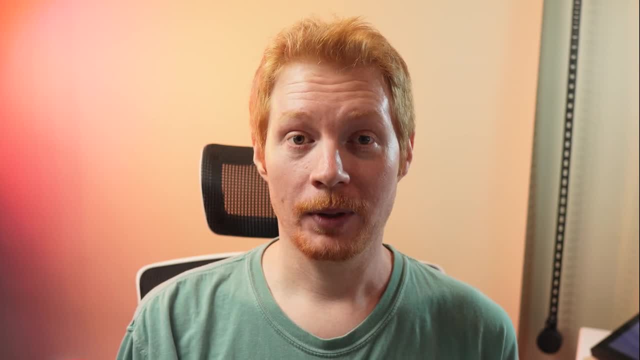 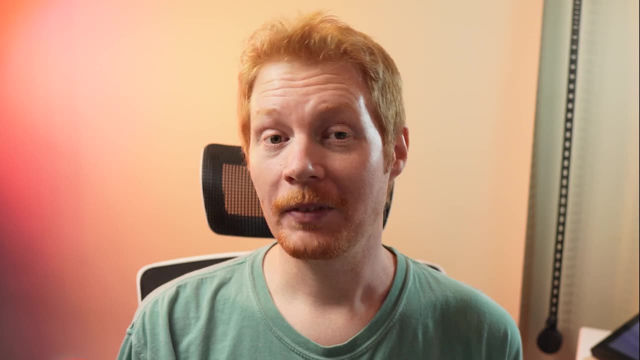 Also, when making changes to your game, keep the same number of components. If you don't, you'll notice that the card art and text are split between each card awkwardly. Hopefully, if you run into that issue, you'll remember this bit in the video.